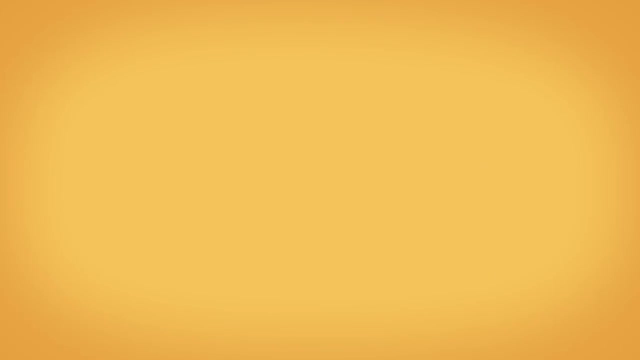 It's important that all online chat customers receive a friendly and positive greeting, but it's also important they receive a response quickly, as quickly as they would if they called you. Customers initiating an online chat will have already experienced a delay whilst their message is transferred to an agent, so it's fine for that agent to shortcut the time it takes to. 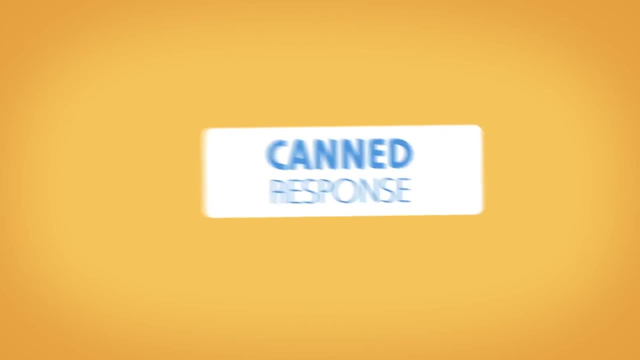 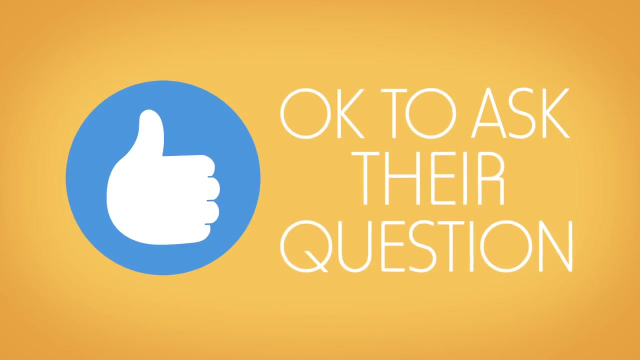 type a greeting by using a canned response. The key here is to ensure your canned responses are genuine, suit your company image and suit the situation. This basic response simply confirms an agent is available and lets the customer know it's okay to ask their question At times. 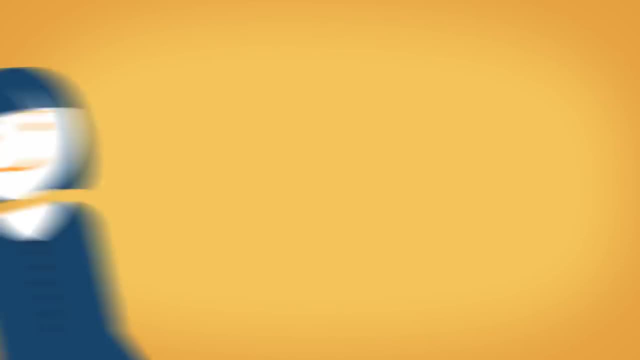 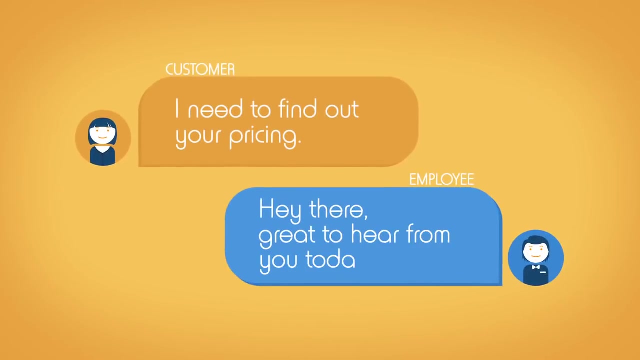 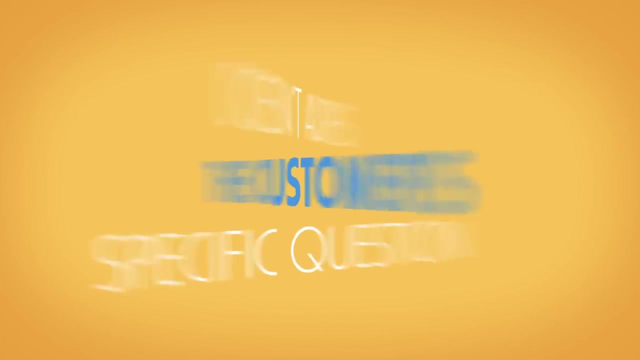 a canned response will not be appropriate, especially when online chat users skip the formalities and get straight to the point. This canned response isn't appropriate. It's clearly an automated response that doesn't address the customer's specific needs- It's a specific question- but instead wastes their time. A better response in this situation. 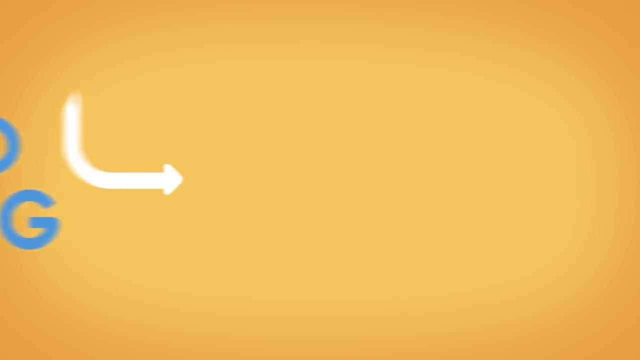 would be to skip the canned greeting altogether and respond with something like: Hi, yes, I can certainly assist with pricing. Which product are you looking at? Canned messages may also be used to shortcut typing out a standard response. This can save the agent typing time, but also saves the agent having to check details themselves. 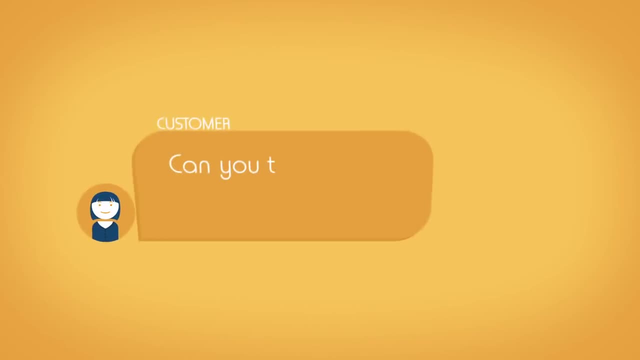 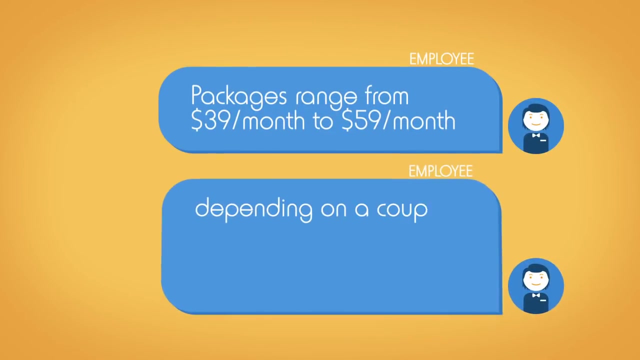 and reduces the risk of error. Can you tell me how much your standard packages cost? Packages range from $39 a month to $59 a month, depending on a couple of variables like how many users you require and which features you need. How many staff do you have? 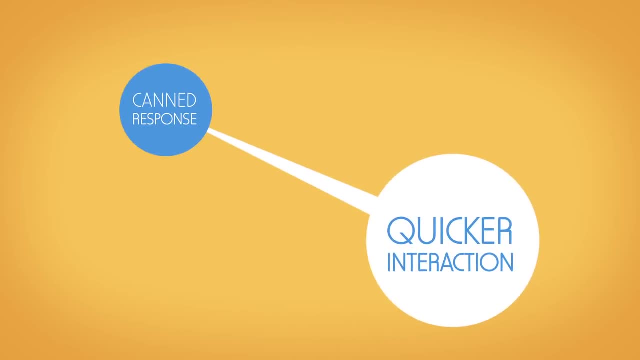 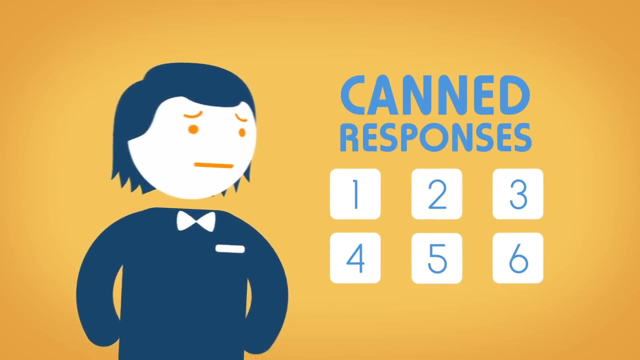 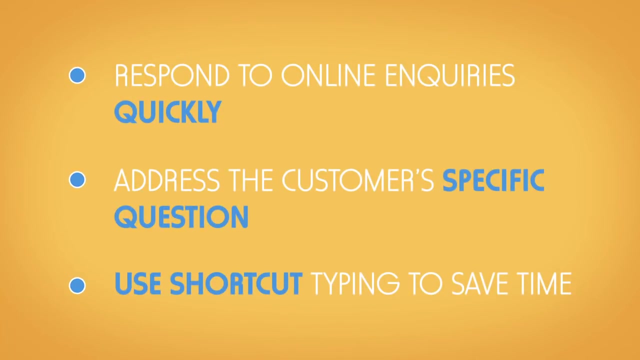 Using a canned response in this scenario made the interaction quicker and also eliminated the chance of making an error. Remember to be selective in your use of canned responses. Don't use them automatically. Use them selectively when appropriate for the situation. Canned messages may also be used to shortcut typing out a standard response. This can save the agent having to check details themselves and reduce the risk of error.